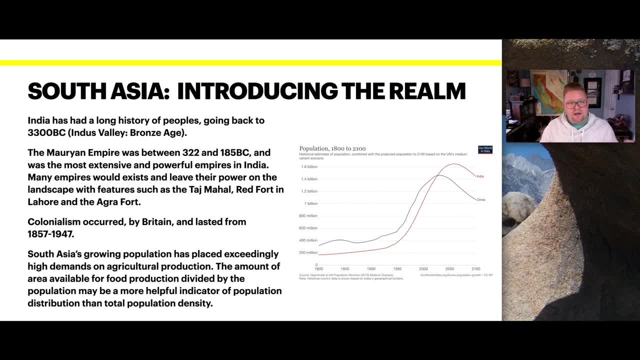 Valley Bronze Age time. The Marayan Empire was between 322 and 185 BC and was the most extensive and powerful empires in India. Many empires would exist and leave their power on the landscape, with features such as the Taj Mahal, the Red Fort in Lahore and the 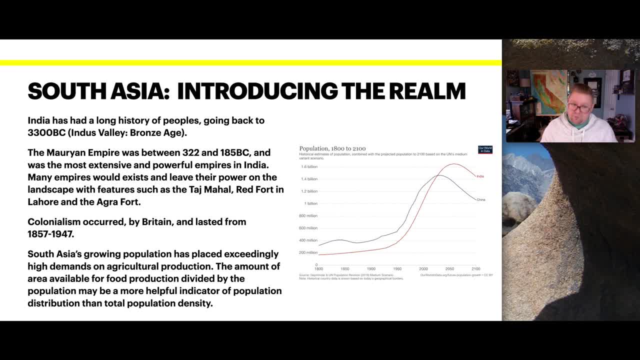 Agra Fort. Colonialism did occur by Britain and it lasted between 1857 to 1947.. South Asia's growing population has exceedingly high demands on agricultural production. The amount of area available for food production is divided by population may be more of a. 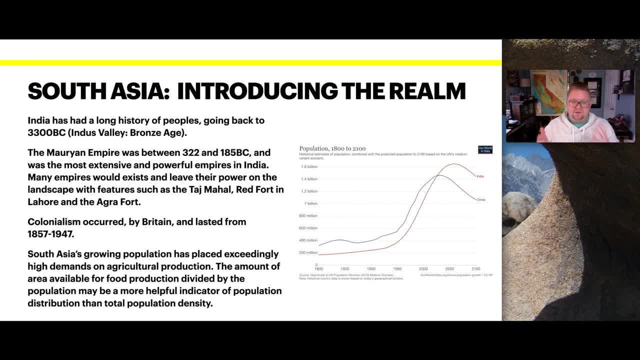 helpful indicator of population distribution than the total population density itself. So, as an example, looking at the diagram on the right hand side, we can see the population over the last well since 1800, so over 200 years. both China and India. We can see that. 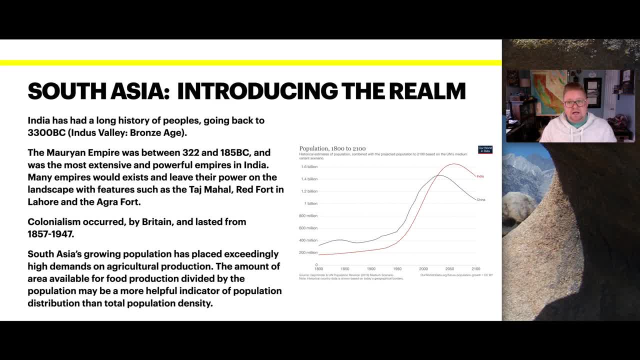 for a long time, even up until the late 1990s, that China was the leading population. Well, but enter now into current time and going forward. it is estimated and has been seen that India has an exceeding population 007. 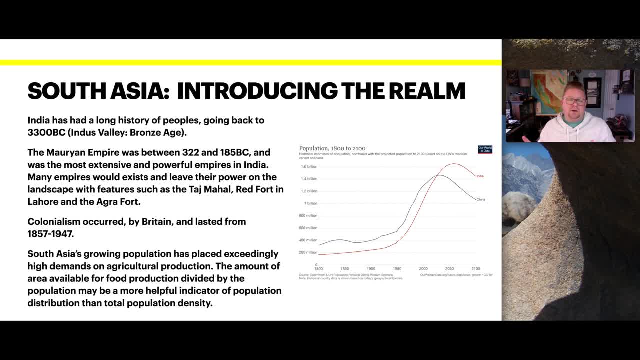 is is growing beyond the, the unfortunate, the death rate right. so you have this balance of how many people are coming in versus how many people are going out, and they are exceeding that, that population volume, which is also turned into concerns of limitation of childbirth, which is we've observed in China with 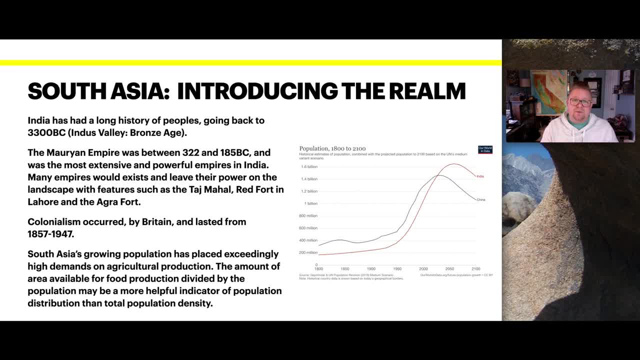 the how many children are you allowed to have, and by putting government regulations and stuff like that. there were some interesting conversations about India and within their caste system and more in the religious peripheral, in how, when a family member dies, who's allowed to bury them? and one 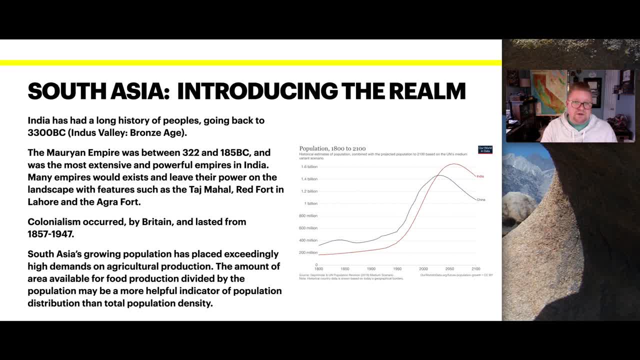 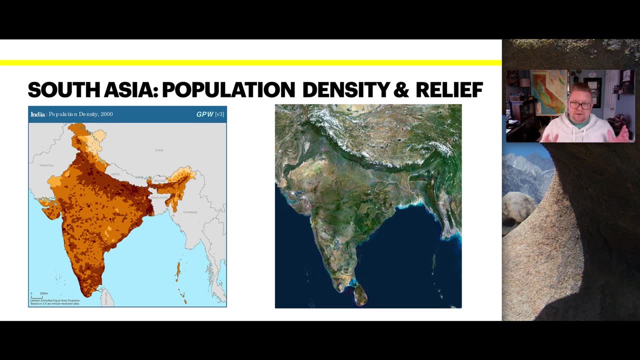 of the cultural aspects, it was you had him, a son, that would bury you, and so a lot of families, if they were having additional females, that they would either have to abort or have to find a way to conceive a son. now looking at the population density and relief, so again side-by-side. 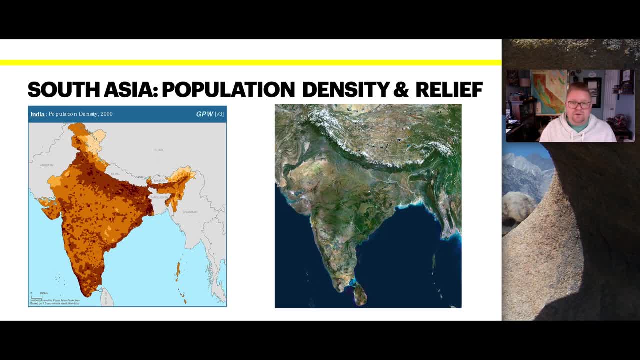 images. population density on the left-hand side raised relief on the right so you can see some of the tallest mountain ranges right there, right you know, along Nepal and Bhutan or whatever. but looking at the population itself, we see again where our populations most dense. they're, in this case, or more dense. 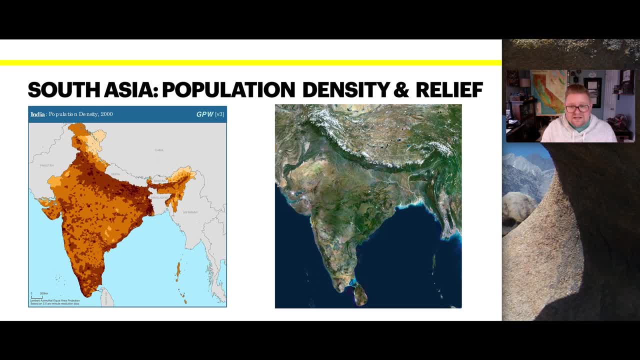 along the peripheral, along the waterways, until you get up into right beneath Nepal. well, why would that be? wait, imagine again talking about just water. we know that agriculture is of dire importance this realm, so people live near where they work and so, since there's still a lot of people that 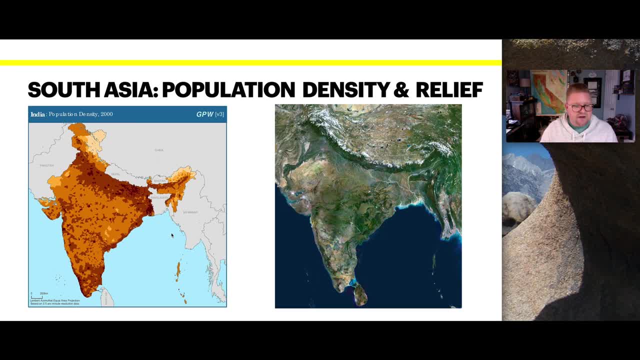 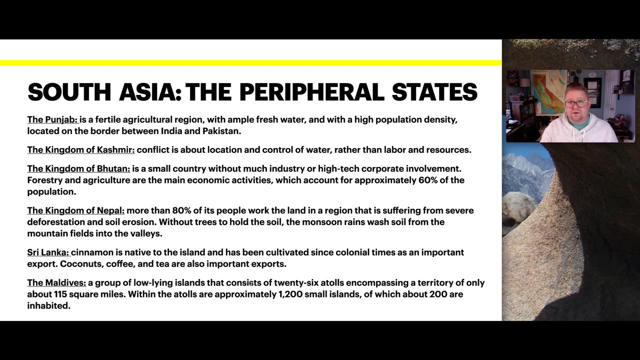 are dealing with agriculture. we find that the density of population is very heavy in the north and also for trade, business and industry down to the south. but we do see again correlations with relief resources and where the density of the population will live. now there are some peripheral states of this realm of south asia. the punjab is a fertile agricultural region. 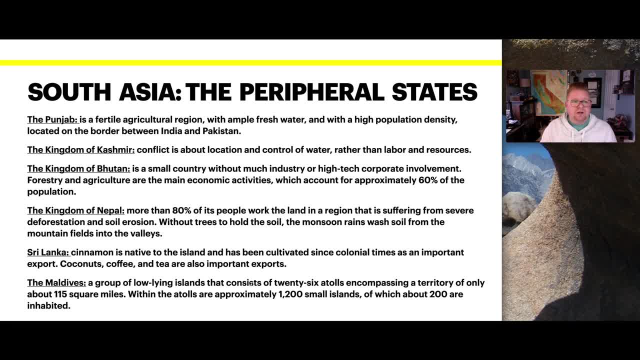 with ample fresh water and a high population density, located between the border of india and pakistan. the king of kashmir conflict is about location and control of water, rather than labor and resources. so they there is no great demand for labor and resources, because without the resource. 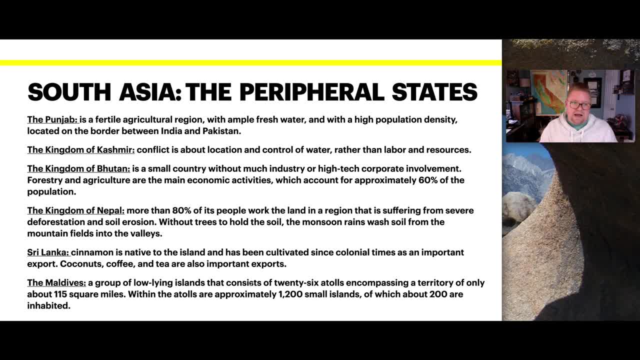 of water alone, you cannot have agriculture, you cannot have industry and you cannot have a population that can survive and grow. the kingdom of butchery town is a small country without much industry or high-tech corporate involvement. forestry and agriculture are the main economic activities, which account for about 60 percent of the population. 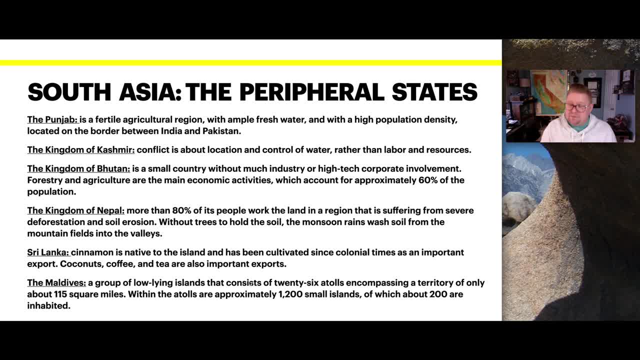 workforce the kingdom of nepal. about 80 percent of those people work in work the land in a region that is suffering from severe deforestation and, as a result, soil erosion because of the deforestation and lack of trees to retain and hold that soil. the monsoonal 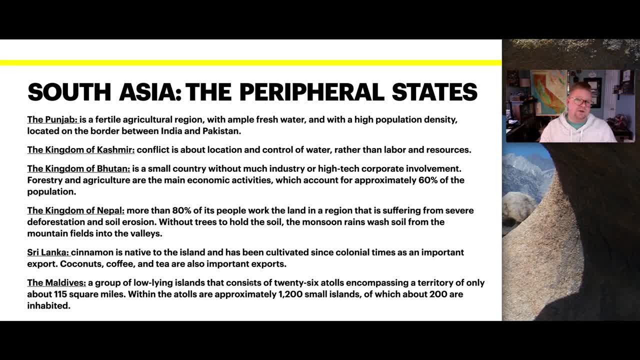 lands will wash that fertile top layer. usually the o horizon or the a, which is the top soil itself, will actually wash it away from the mountain fields into the valleys. sri lanka cinnamon is native to the island and has been cultivated since colonial times as its most important export, still to this day. but on top of that, coconut, coffee and teas are. 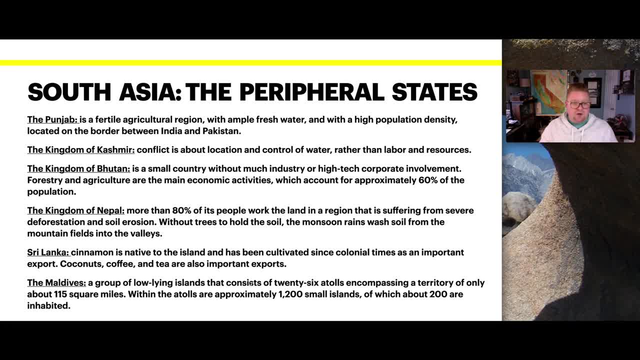 also very important financial exports. the maldives, a group of low-lying islands that consist of about 26 atolls, which atolls are the remnants of volcanic- oceanic volcanoes that had completely eroded and left behind just the rim, which encompass a territory of about 115 square miles. within the atolls, about 1200. 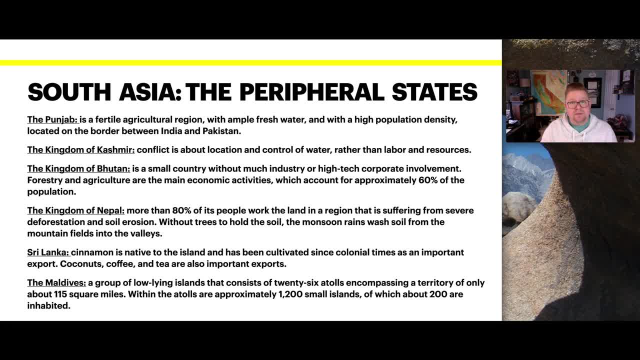 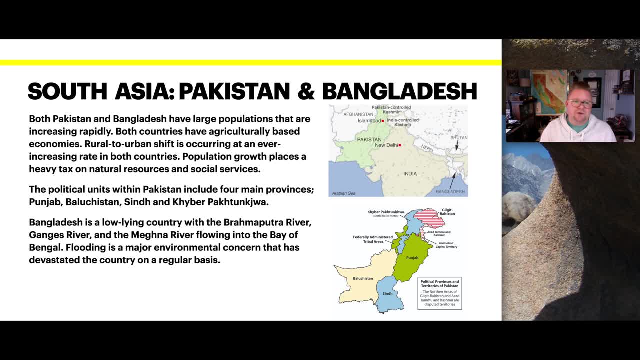 smaller islands, of which about 200 are inhabited by people. now we'll also include pakistan and bangladesh. so both pakistan and bangladesh have very large populations that are increasing rapidly. both countries have agricultural and cultural-based economies. rural to urban shift is occurring at an ever-increasing rate in both. 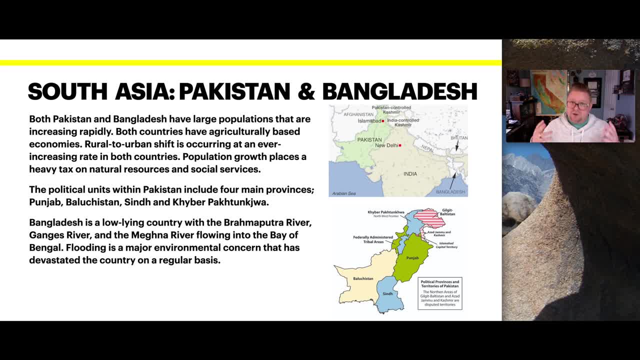 those countries and population growth places an incredible heavy tax on natural resources and social services. the political units within pakistan include the four main provinces: punjab, balochistan, sin and the khyber. bangladesh is a low-lying country in which the dominant river, actually the ganges in particular, flow into the bay of bengal. 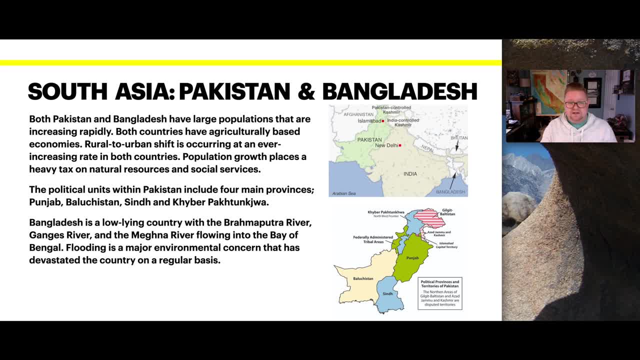 flowing is. flooding is a major environmental concern that has devastated the country on a regular basis, but we also find that flooding can also be important in areas in the release of nutrients. but again, dealing with the monsoonal rains, sometimes the rate of erosion is exceeding that of deposition, and so it does become quite troublesome. 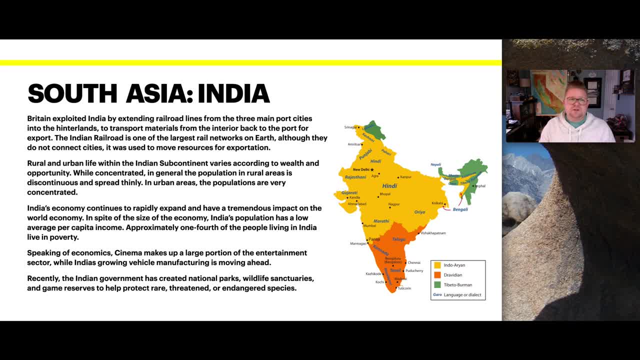 so let's look specifically at india for a moment. so britain exploited india by extending railroad from the three main port cities into the hinterlands to transport materials from the interior back to the port for export. the indian railroad is one of the largest rail networks on. 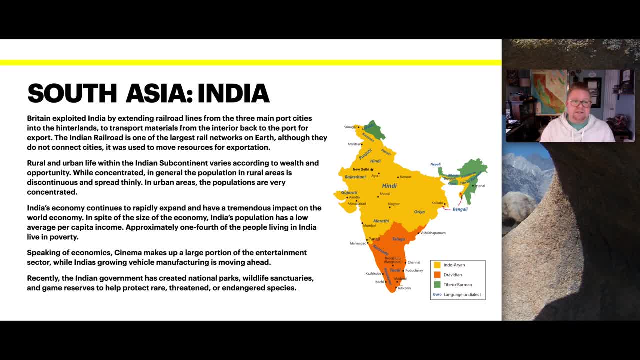 earth. although it does not connect major cities, it was used to move resources for exportation, which is really interesting. so there's this. you know, one of the largest railways in the world is observed here and it wasn't designed for people to bring people together in transportation. it was specifically to exploit the export. 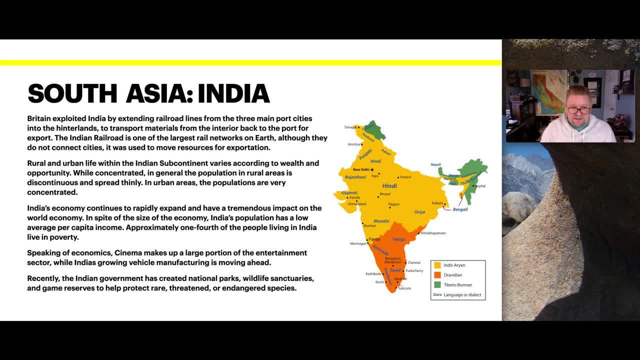 of goods and services and transports. rural and urban life within india subcontinent varies according to wealth and opportunity. while concentrated in general, the population in rural areas is discontinuous and spread quite thinly, in urban areas the populations are very concentrated, so again that rural to urban shift is very prominent. india's economy continues to rapidly. 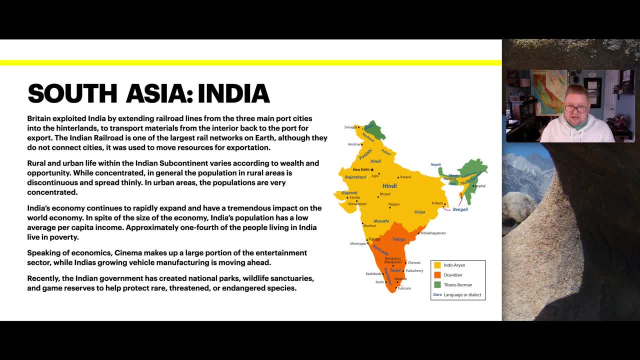 expand and have a tremendous impact on the world economy itself. in spite of the size of the economy, india's population has a low average per capita income. approximately one-fourth of all people in india are living below poverty. now, speaking of economics, cinema makes up a very large portion. 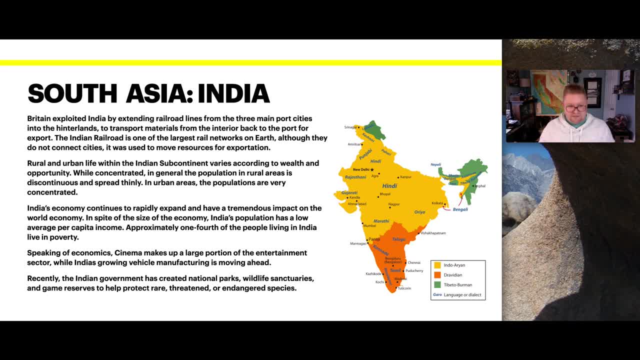 of the entertainment sector and part of its financial sector, while india's growth via, so while india's growing vehicle manufacturing is actually moving ahead progressively. recently, the indian government has created national parks, wildlife, sanctuary areas and game reserves to help protect rare, threatened or endangered species. the diagram: 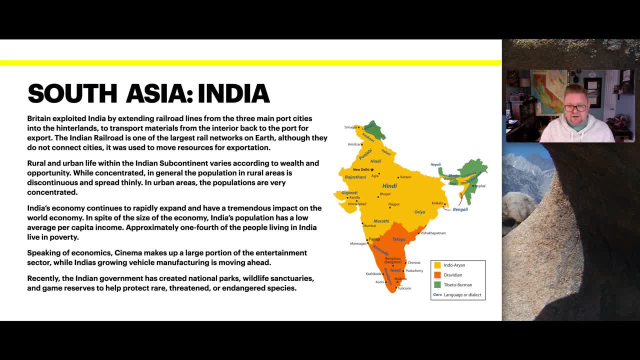 that i chose for the right is showing some of the language distribution. i guess that would be an interesting way for you to then. if you want to look at this and then shoot back into population densities, do we find that there are certain populations that are more prone to speak this? 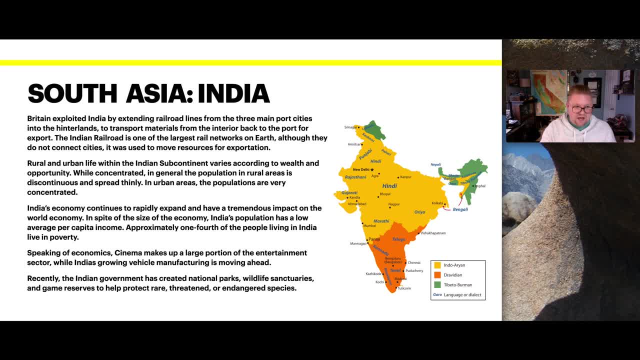 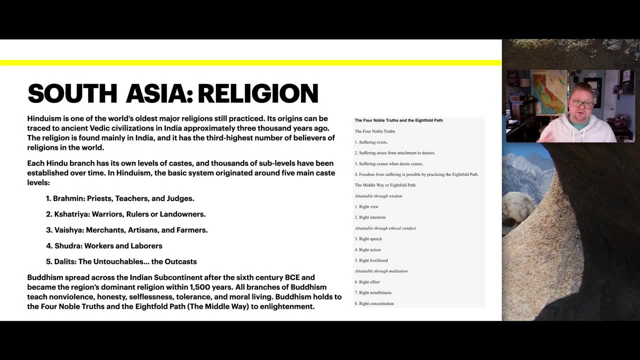 parent language. you know lingua versus others, which brings us into religion. hinduism is one the world's oldest major religion still being practiced today. its origin can be traced back to ancient vedic civilizations in india, approximately 3 000 plus years ago. the religion is found mainly in india and has the third highest number of believers in any religion. 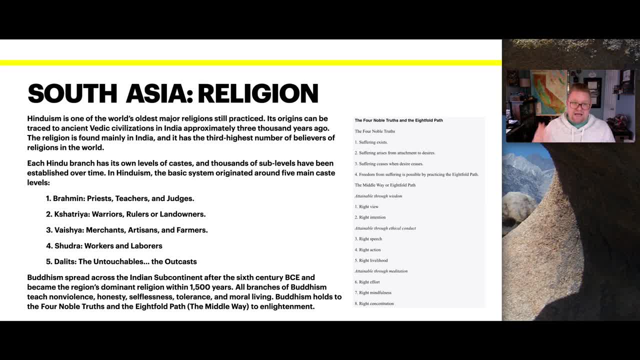 in the world. each hindu branch has its own level of casts, and thousands of sub-levels can be established over time within those. in hinduism, the basic system originated of the five main caste levels. so what's interesting about the cast level is it's born. 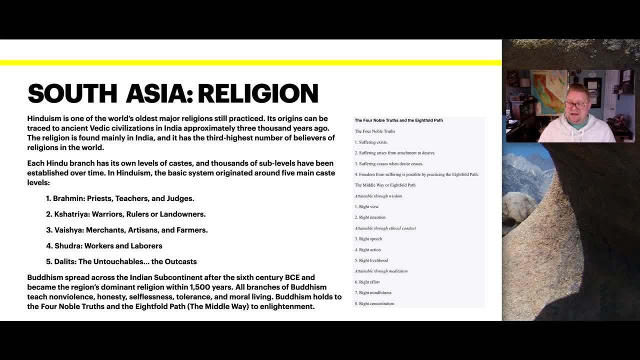 into. it has nothing to do with how, how hard you work, how, how not hard to work, things like that. it's a system that you're born into. so you you're born into being a priest or teacher, born into being a warrior or a merchant or a laborer or what's considered the untouchables or outcasts. 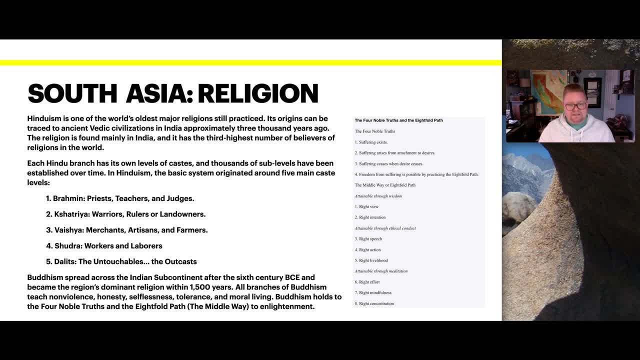 buddhism spread across india subcontinent about the 6th century bc and became the religion's most dominant religion within 1500 years, when the indian kings of india took over the indian religion. within years, all branches of buddhism teach non-violence, honesty, selflessness, tolerance and moral living.